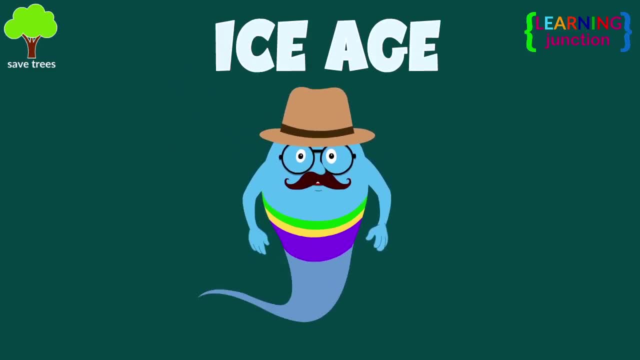 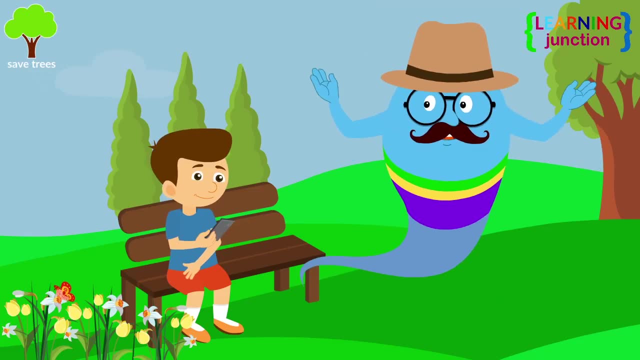 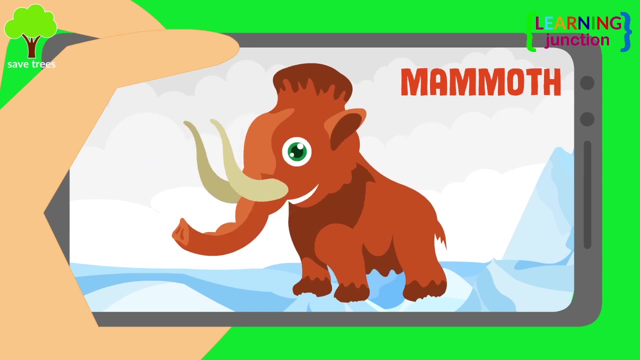 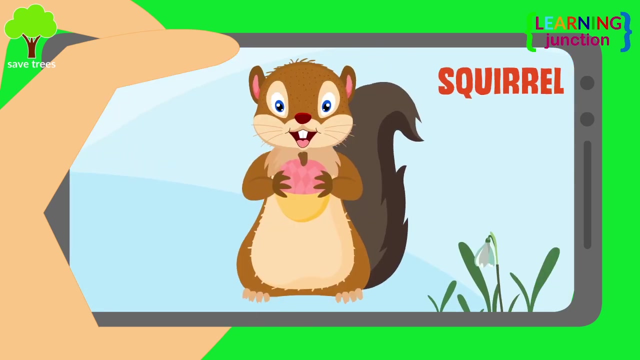 Hello friends, Today we'll learn about the Ice Age. Oh, you're watching videos of these Ice Age animals. Show it to your friends. Look at this giant mammoth, So huge. Ah, this one is a saber-toothed tiger. This squirrel looks so different. 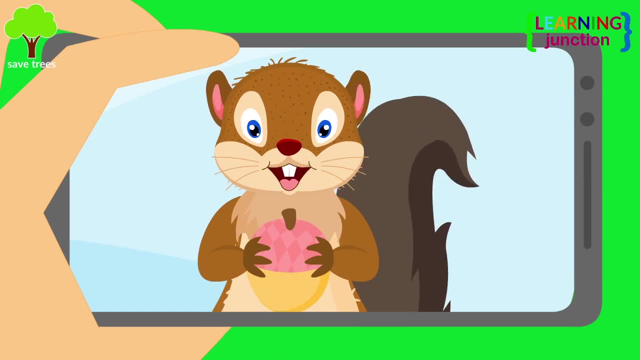 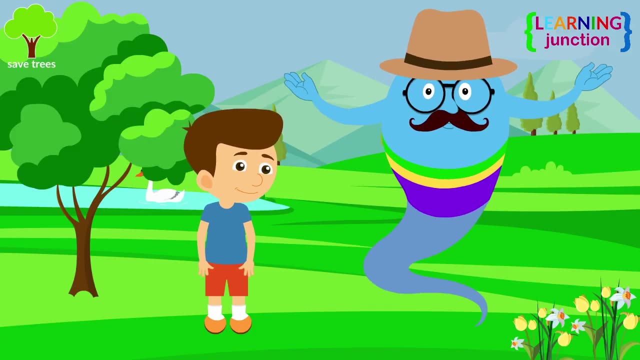 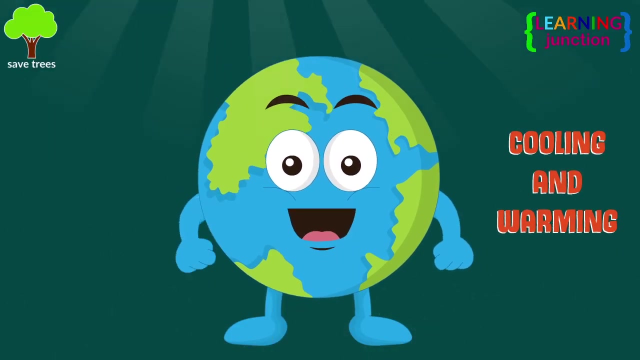 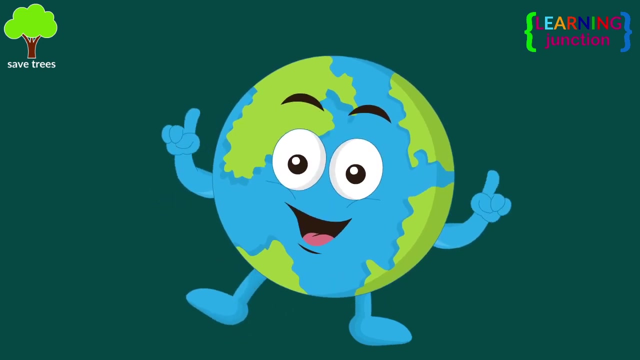 from today's squirrels, Zoom into this. Very cute, isn't it? Are you ready to explore all about the Ice Age? Let me explain it to you. Planet Earth has experienced several periods of cooling and warming episodes throughout its history. The Ice Age is a period in the Earth's history that began approximately. 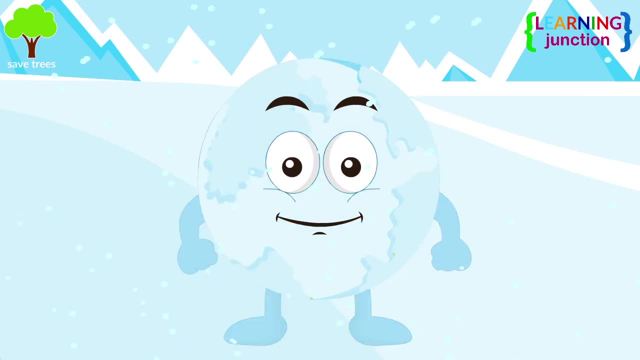 70,000 years ago. It was the time when most of the Earth's life began. It was the time when most of the Earth's life began. It was the time when most of the Earth's life began. It was the time when most of the Earth's 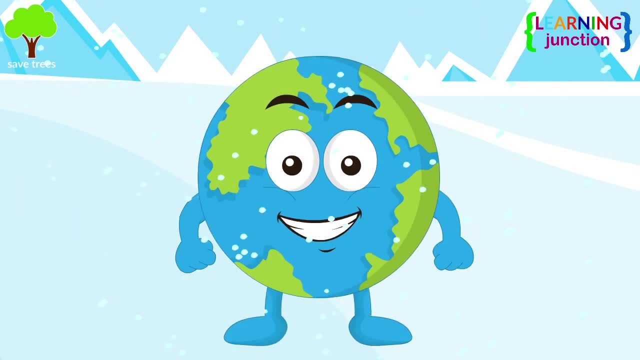 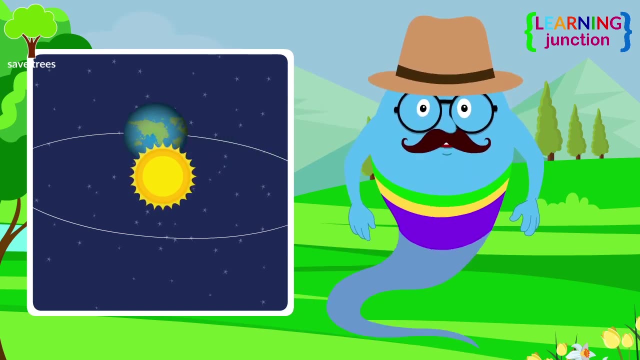 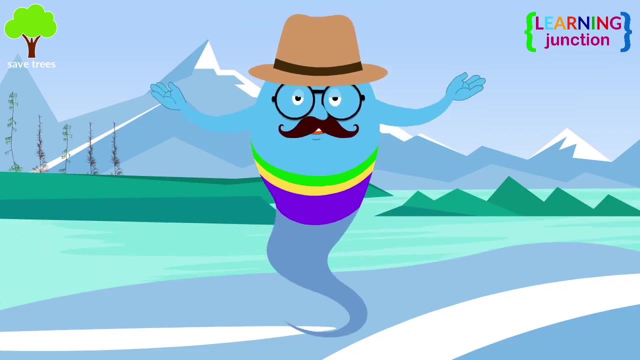 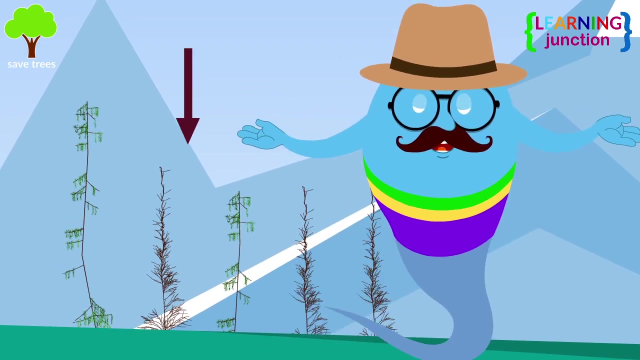 surface was buried under thick sheets of ice. Most geologists believe that the ice ages are convicted by a chain reaction of positive feedbacks triggered by periodic changes in the Earth's orbit around the Sun. During the Ice Age, the Earth's surface was entirely frozen. Only a few plants, including the 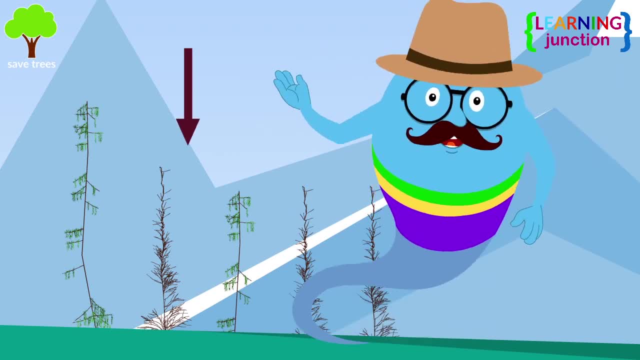 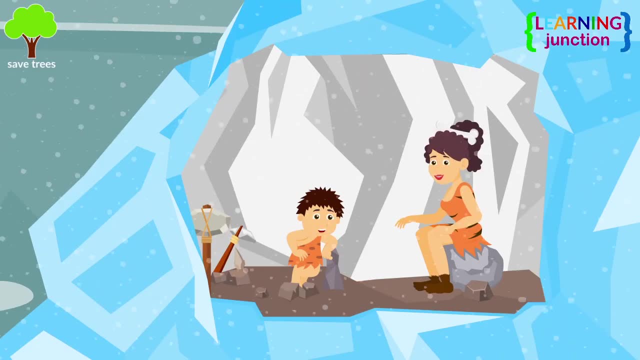 evergreen trees could grow in the harsh, frozen soil. There wasn't enough carbon dioxide in the air to support vegetation. The analysis showed there were humans in North America before, during and immediately after the peak of the last Ice Age. Population was very less because it was so tough to 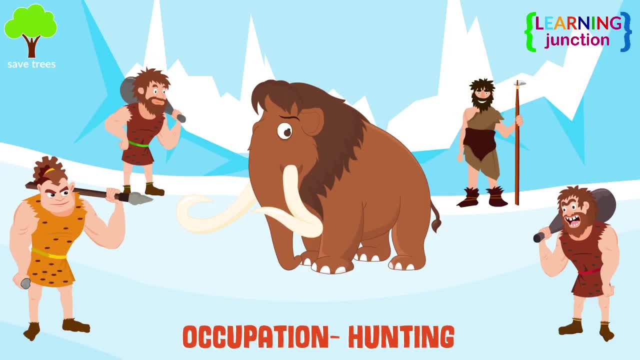 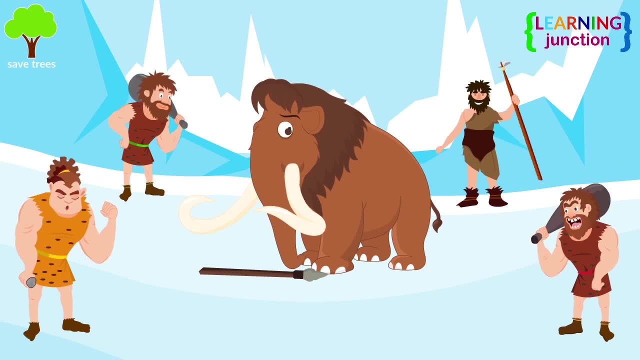 survive an extreme cold. The main occupation during that period was hunting. They used to travel long distances and search for food and shelter For hunting. they had to hunt for food and shelter For hunting. the hunting: they used to travel in groups. People used to wear the animal's skin to. 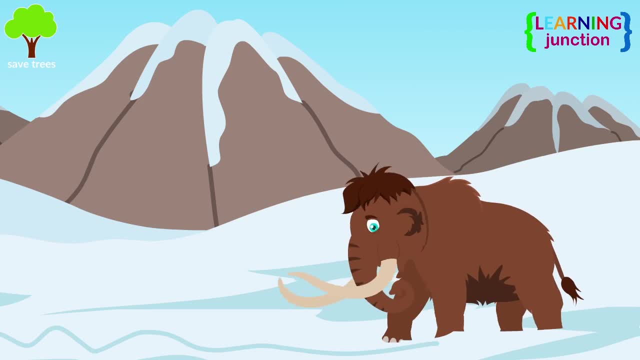 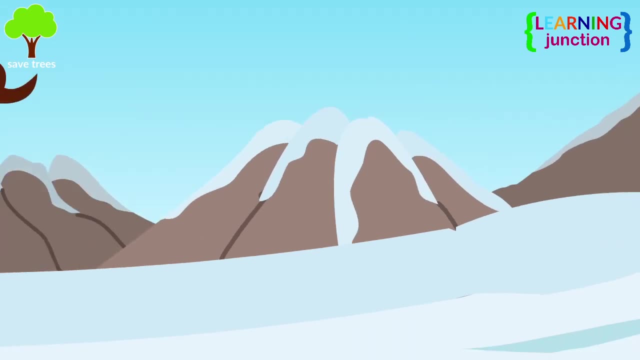 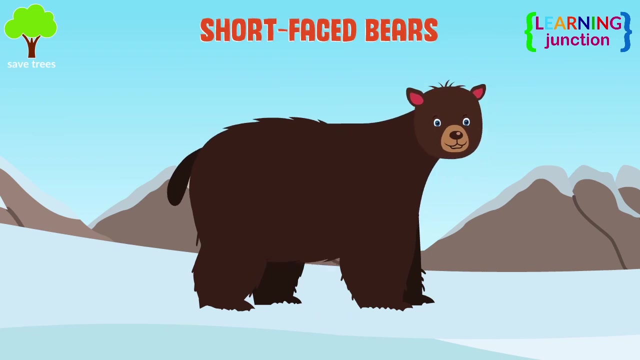 stay warm. Some of the important animals of those times were the woolly mammoth, very, very dangerous dire wolves, some species of Irish Elks and the giant bears. Ice Age short-faced bears were the largest mammalian land carnivores to. 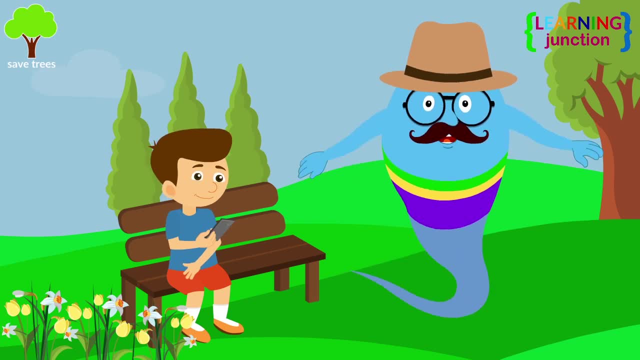 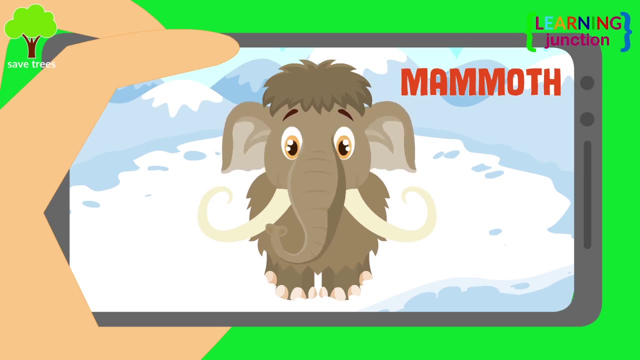 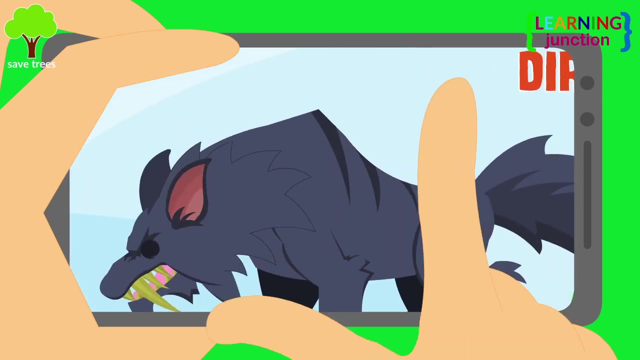 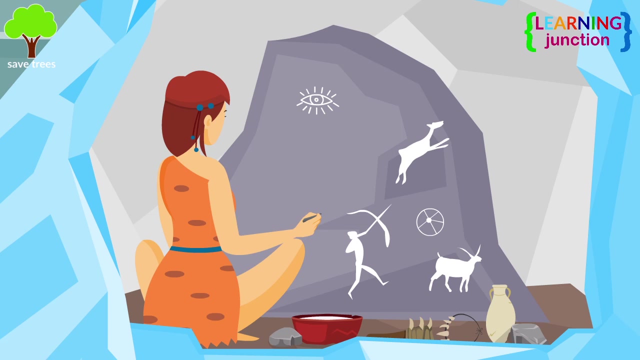 ever live in North America, closely here buddy. huge multi-ton animals like mammoths disappeared, along with apex predators like saber-tooth tigers and dire wolves. dire wolves were fearsome predators. people used to draw the pictures of animals and various other things on the walls of their caves. 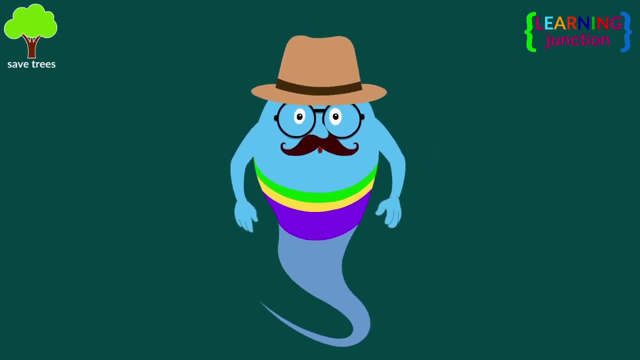 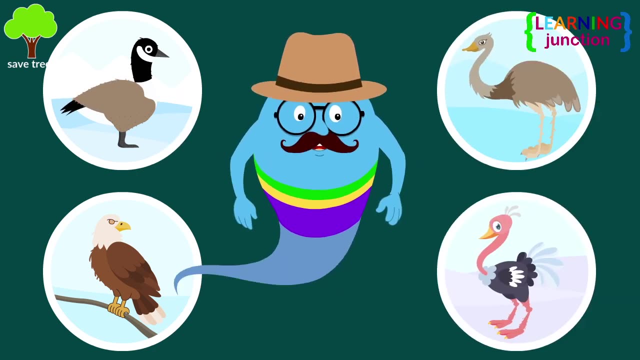 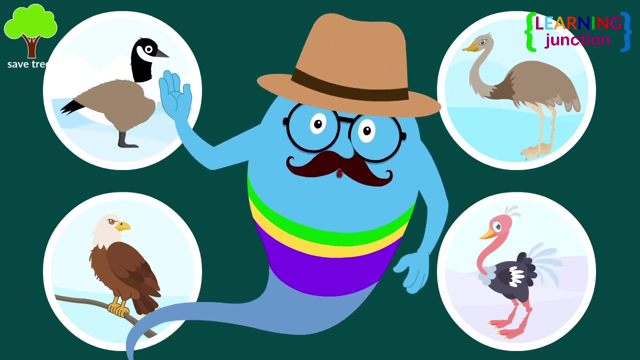 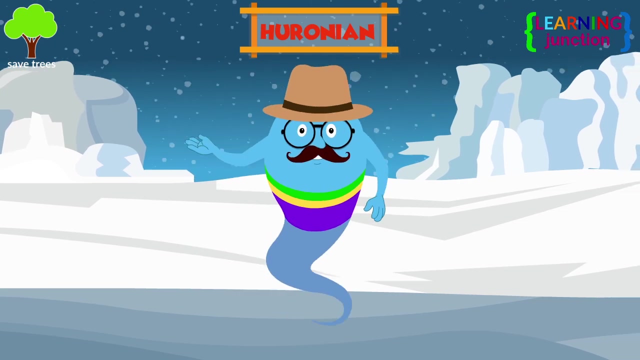 birds flourished during this period, including members of the geese and eagle families. there were also some flightless birds, such as rias and ostriches. the earth has experienced five major ice ages. let's study about these one by one. huronian: this was one of the longest ice ages in the earth's history. it lasted from 2400 to 2100. 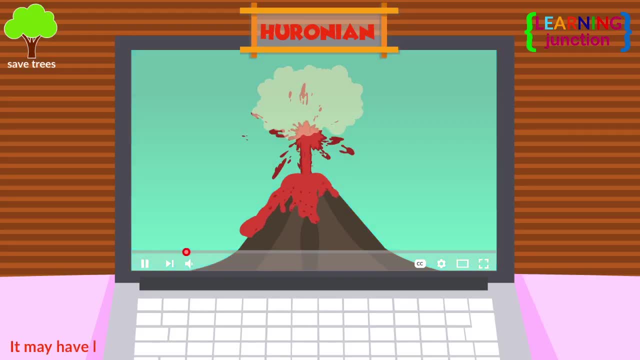 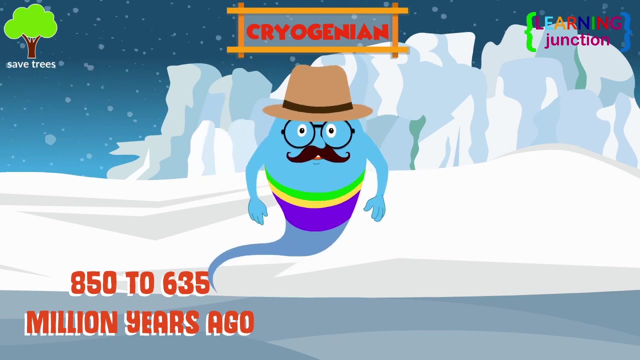 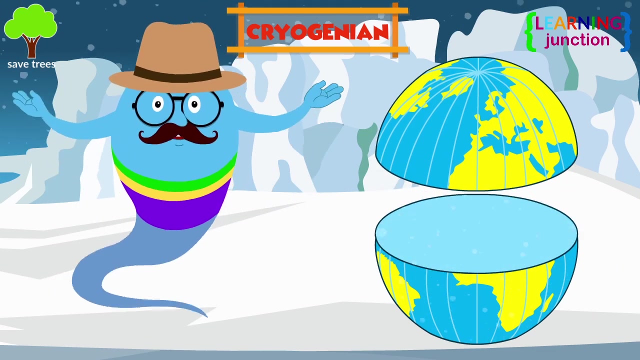 million years ago. scientists think it may have been caused by a lack of volcanic activity lowering the carbon dioxide in the earth's atmosphere- cryogenian. this ice age occurred from 850 to 635 million years ago. it is possible that ice sheets reached all the way to the equator. 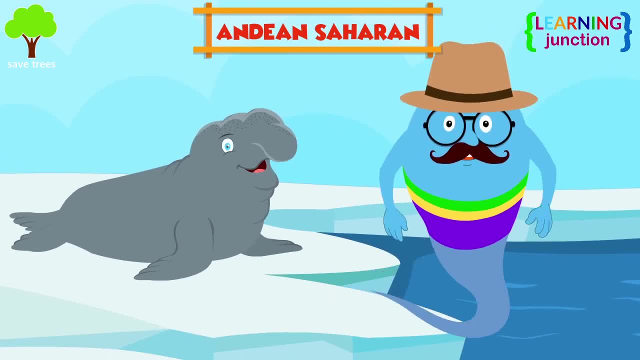 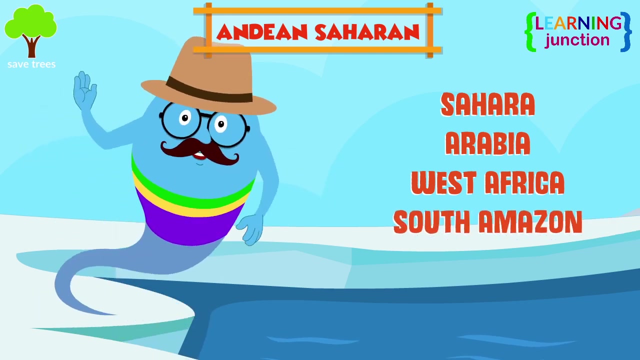 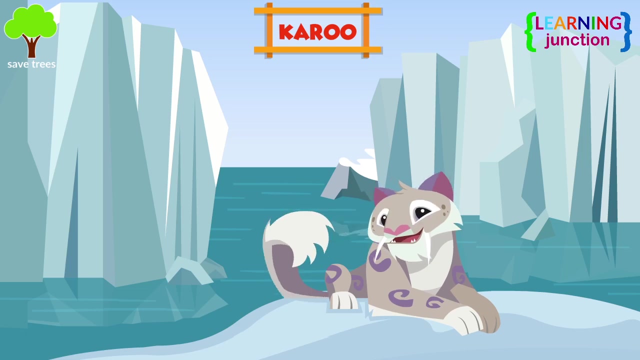 andean saharan. the andean saharan ice age occurred between 460 to 430 million years ago. during this age glaciation is known from sahara, arabia, west africa, the south amazon and the andes karu age. this ice age lasted around 100 million years, between 360 to 260 million years ago. 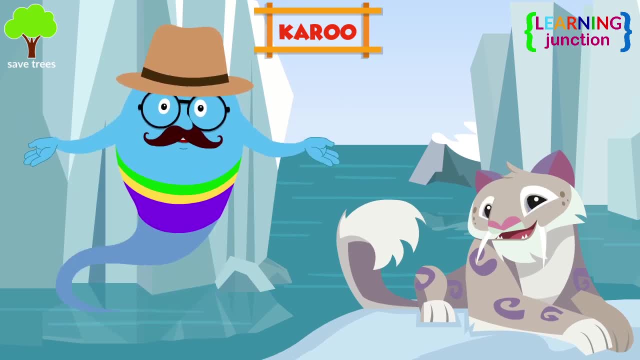 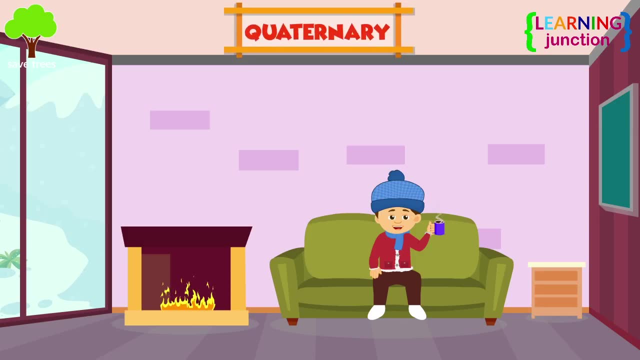 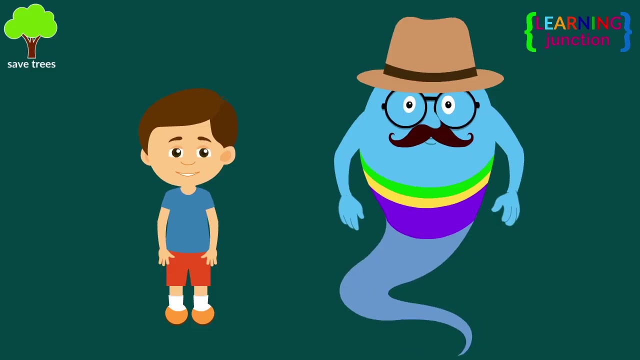 it is named after glacial tills in karu, south africa, that geologists think were developed during this period. you may be surprised to know that we're currently living in an ice age, called the quaternary ice age. it started approximately 2.5 million years ago and is still going now. 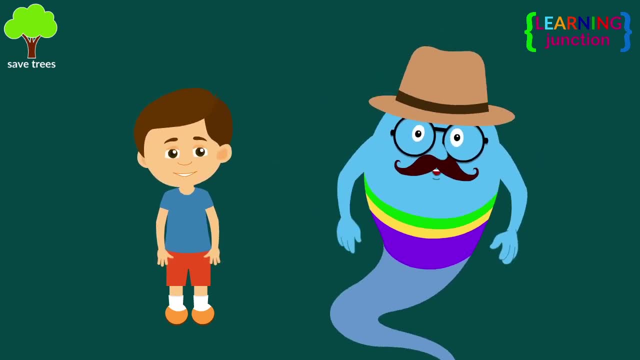 you know a lot about the ice age. stay tuned for more videos. bye, bye.